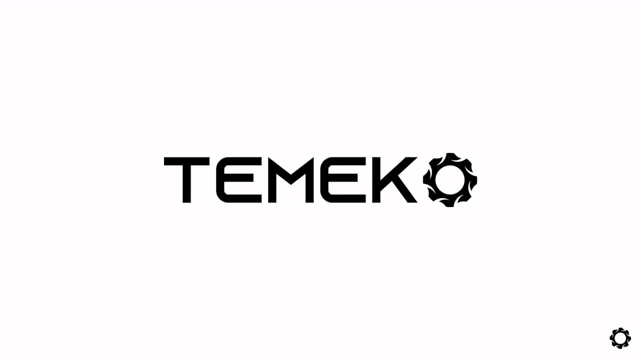 Hi and welcome to Temeco. In this video, we will talk about constraint equations. This doesn't sound familiar, and it's not because constraint might not be a word that we use so often. However, in our case, multibody dynamics modeling heavily relies on constraints, and how. 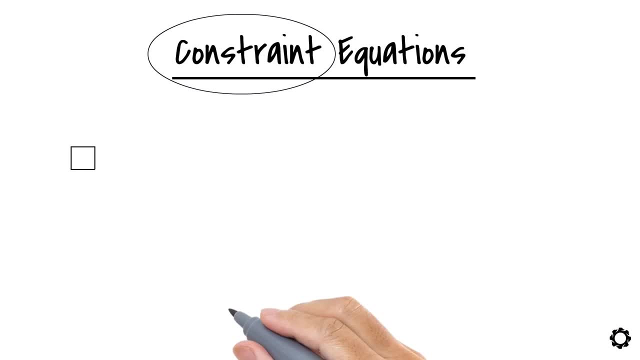 we approach them. In this video, I plan to introduce you to the concept of constraint equations and I will share with you why it is so important in modeling physical systems. Bear with me, Let's recap. In one of our introductory videos, we talked about three concepts. 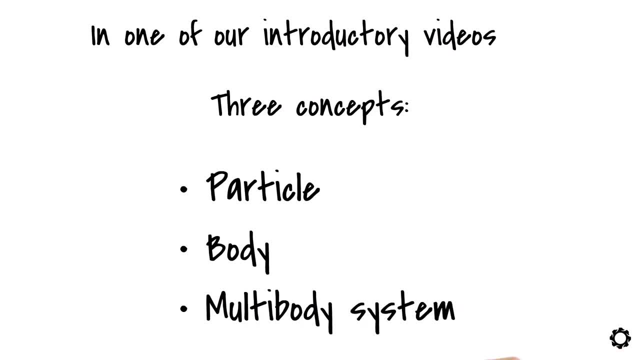 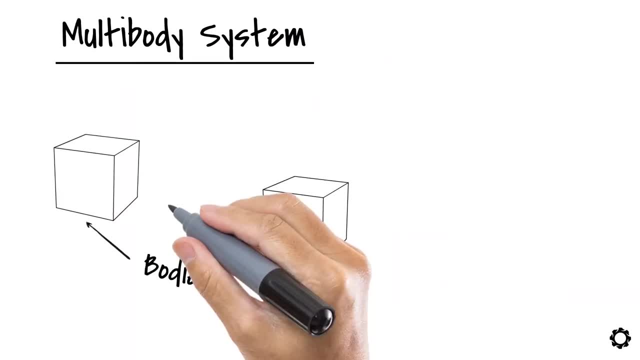 Those were the concepts of particle body and multibody system. The latter is where we are going to focus. We mentioned that a multibody system could be defined as a collection of bodies joined together with constraints, And we also mentioned that this multibody system has a 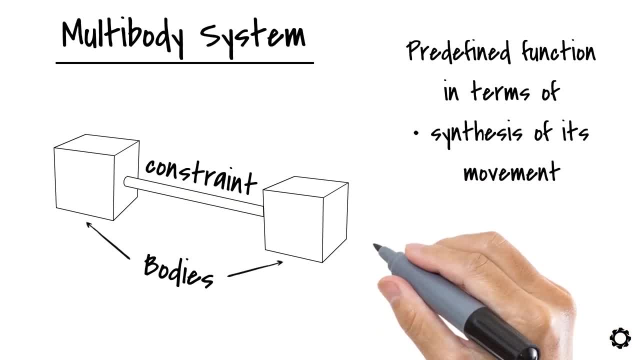 predefined function in terms of synthesis of its movement. Velocities are accelerations of certain body parts. Exerts a specific force to another object- You name it Now. to accomplish this function, besides the dimensions or general arrangement of the system, important care has to be taken when selecting the constraints to join. 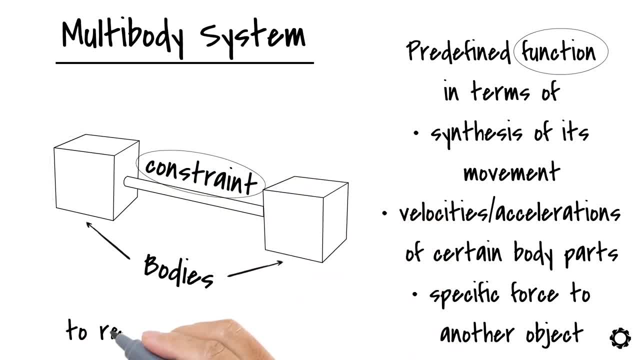 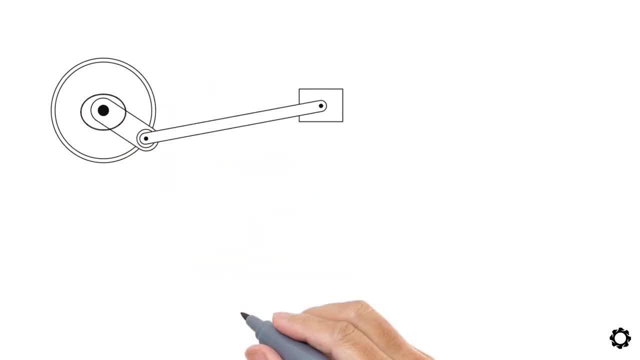 the bodies, because the ultimate job of a constraint is to restrict, to limit the possible relative movement between two bodies. You would use a type of constraint, when you only want one, to allow a relative pure rotation of one body with respect to the other, Or you would use another type of constraint. 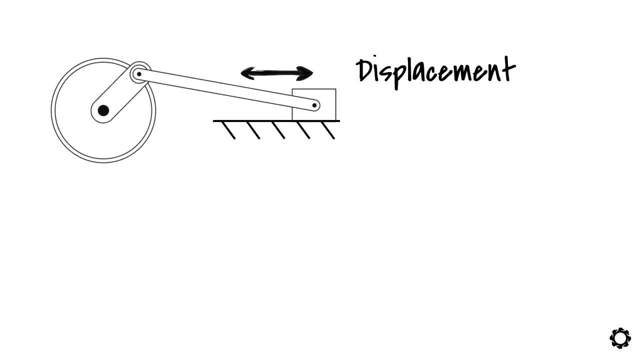 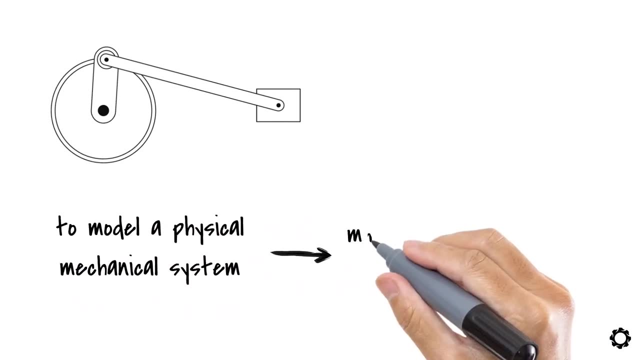 constraint when you only want to allow for a displacement between one body and another. We have also said that to model a physical, mechanical system, we need to be able to describe the system in mathematical terms, And that was basically done with the equation of motion. 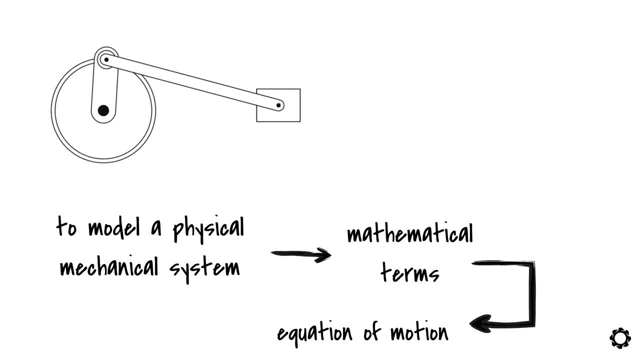 of the system. Well, we need a way to tell mathematically what are the constraints and which bodies they are attached to. I think you're getting the idea of what I'm going to say next. If you thought about constraint equations, you were totally right. Yes, constraint equations. 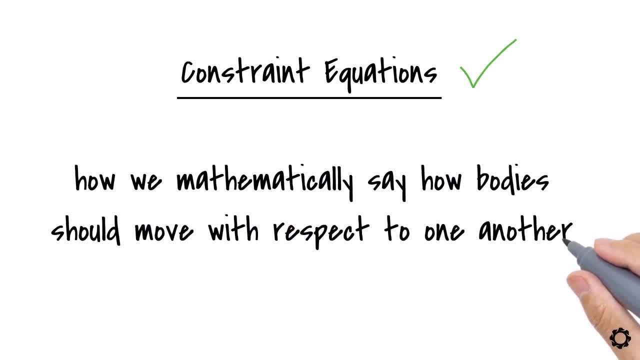 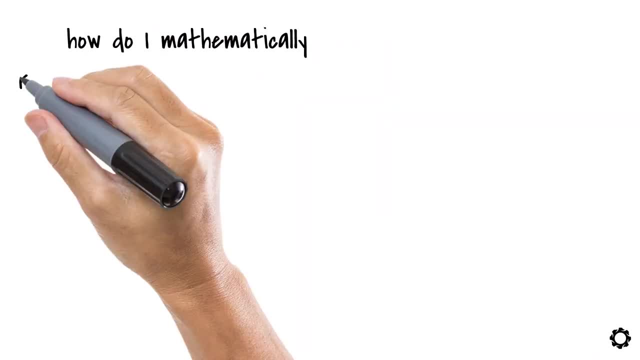 are how we mathematically say how bodies should move with respect to one another. This is the point where our mind could start wandering. You can tell me okay, but how do I mathematically represent a specific constraint such as those you described for the crankshaft mechanism? 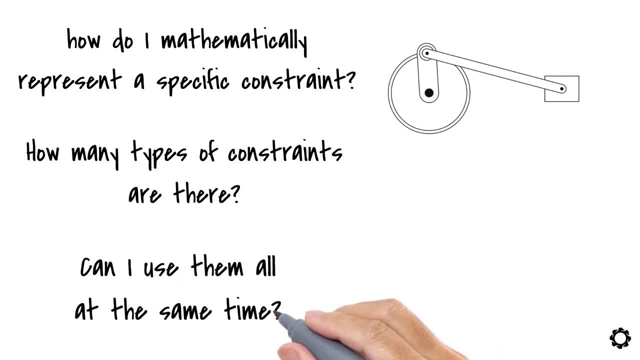 How many types of constraints are there? Can I use them all at the same time? For sure, these and many other questions are popping up in your head. Be patient. If you have any questions, feel free to ask them in the comments section. 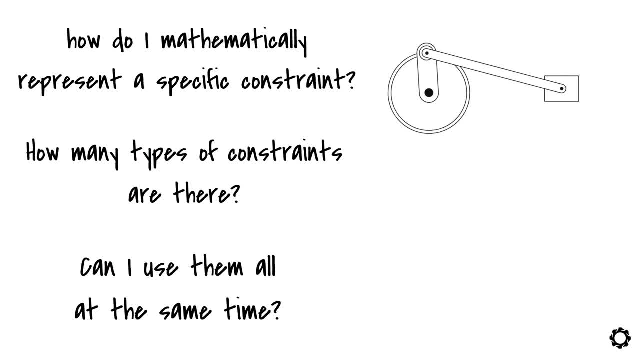 They will get an answer throughout our lessons. The important thing here is that you grasp the concept of having something, a mathematical form of saying these are the constraints used. Let's jump one step back Before going into the details of what type of constraints they. 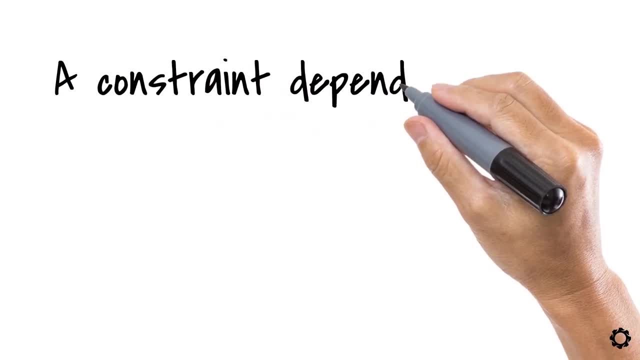 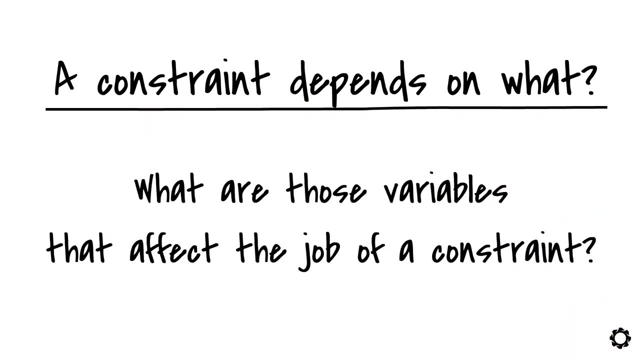 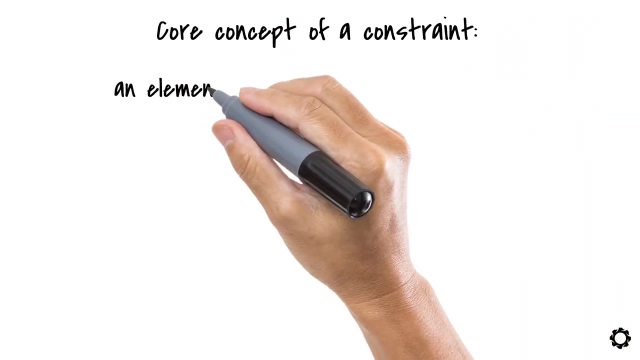 are. I could also ask myself: a constraint depends on what Or what are those variables that affect the job of a constraint in general? I think these are among the first questions that we should tackle If we start with the core concept of a constraint, which is an element that restricts or limits. 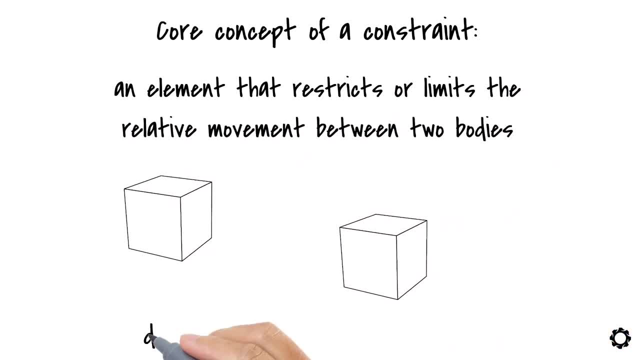 the relative movement between two bodies. I am already talking about degrees of freedom. Each body in space has six degrees of freedom when they are not attached to anything else. As soon as we join this body to another using a constraint, I start restricting degrees. 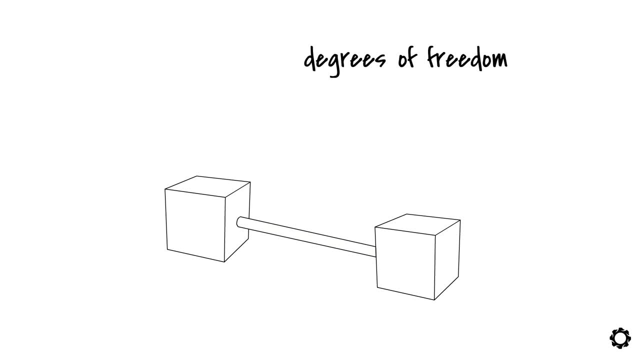 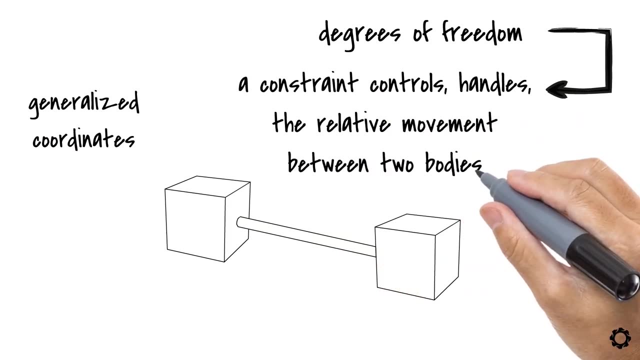 of freedom. Knowing that I describe degrees of freedom using generalized coordinates, then it would be similar to restricting degrees of freedom using generalised coordinates. I would also like to say that a constraint controls handles the relative movement between two bodies by considering which generalised coordinates are available to it to do the 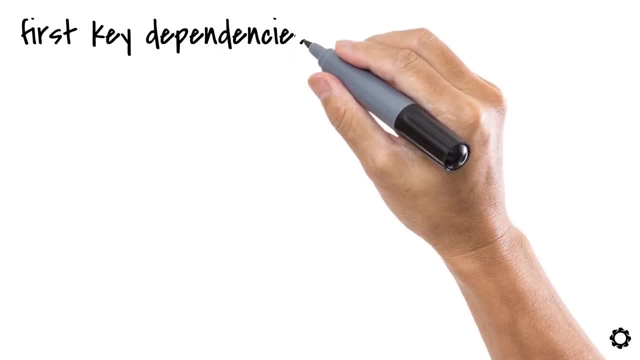 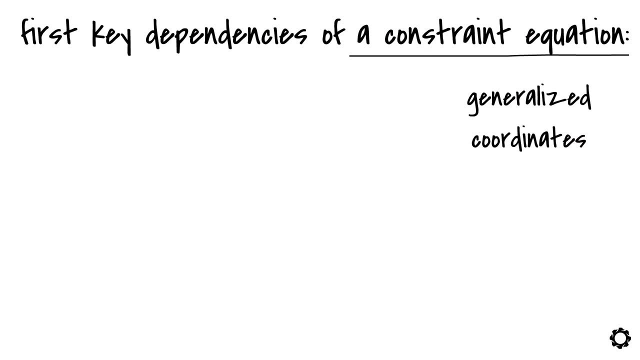 job, We intuitively found the first key dependencies of the constraint equation. That is, a constraint equation depends on the generalised coordinates used to create the model. Mathematicians would write something like: if q1, q2, q3, until qn are each one of our generalised coordinates, and n being the number of total generalised coordinates, we would write q1,, q2, q3, until qn are each one of our generalised coordinates, and n being the number of total generalised coordinates, we would write q1,, q2, q3, until qn are each one of our generalised coordinates. 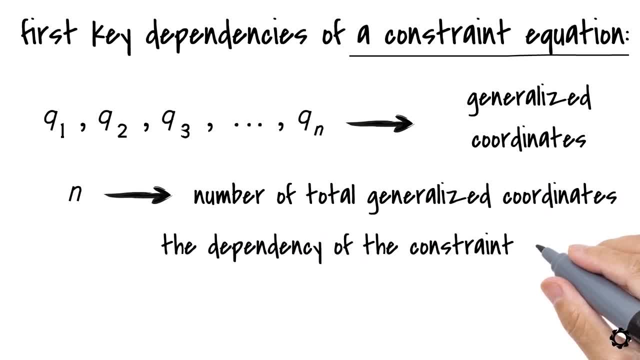 which contains our sequel c, That is, the ability to we continue our exercise just like this. So, instead of creating the instability��고 the constraint equationんだ. this is called Korea's concentration between two bodies. we are doing itawathromebyaking a model, then. 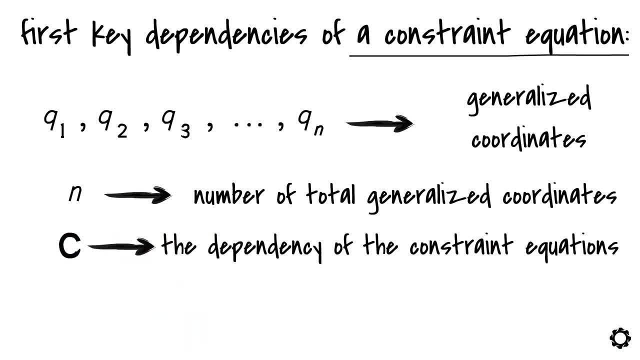 the dependency of the constraint equationsthat I will call from nowon ccan, be written as c of q1, q2, q3, until qn equals 0.. Wait a second. You might say You were sayingthat constraint equations depend on the generalised.